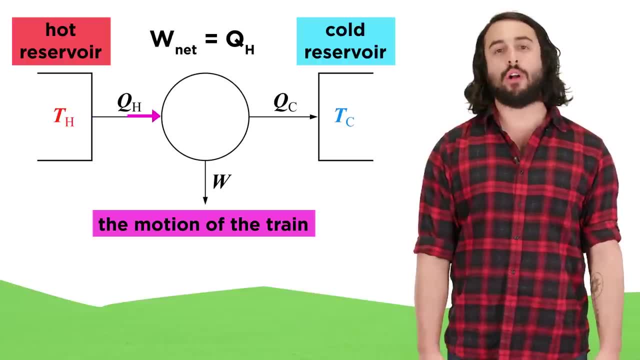 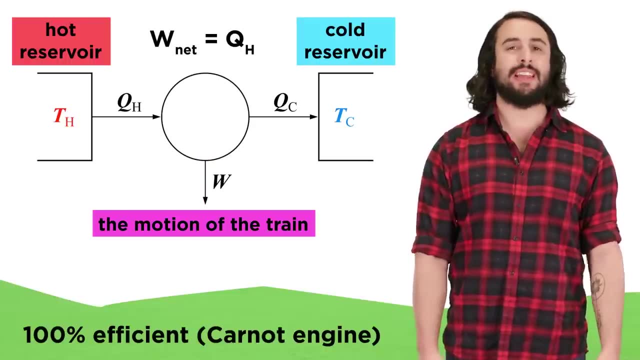 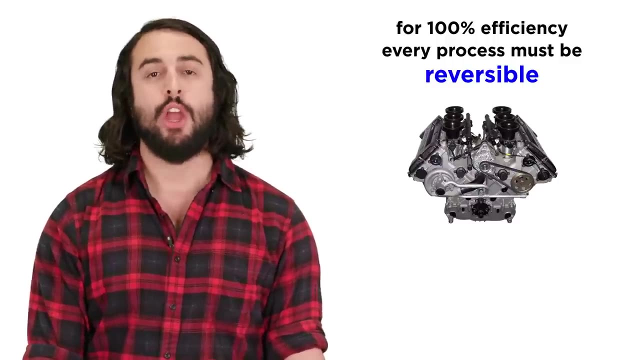 If there was truly zero heat loss, we could say that all of the heat is transferred to work and the engine operates at one hundred percent efficiency. Unfortunately, this is not physically possible for a number of reasons. First, the only way to achieve one hundred percent efficiency would be if every process 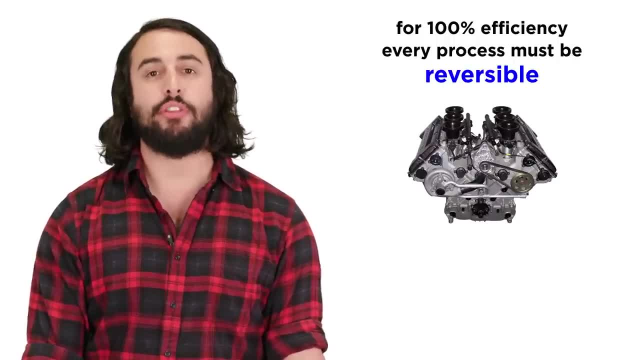 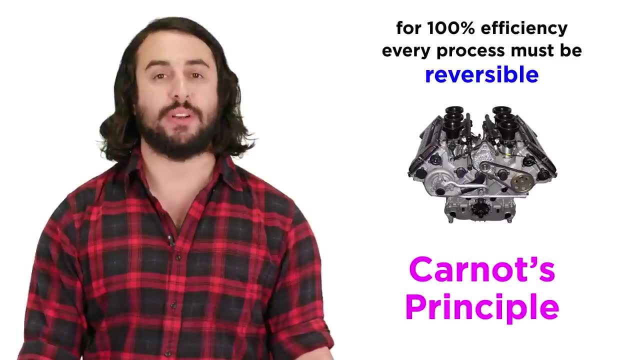 in the engine were completely reversible, meaning both the system and surroundings could return to their original states. This is known as Carnot's principle, but any real engine involves moving parts that produce friction and stress. This is known as Carnot's principle, but any real engine involves moving parts that produce friction and stress. 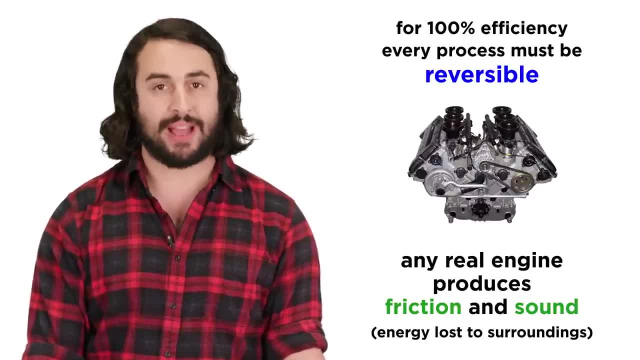 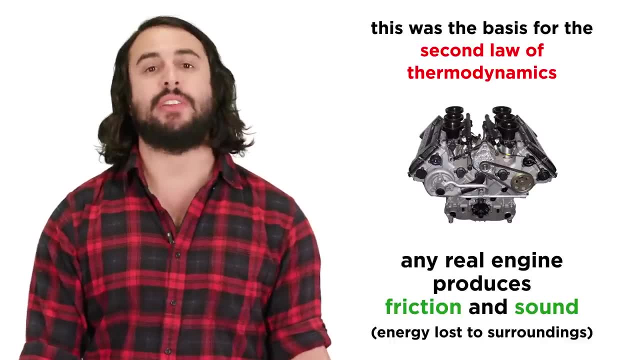 This is known as Carnot's principle, but any real engine involves moving parts that produce friction and stress, So some energy must always be lost to the surroundings. This conclusion does not immediately follow from the first law of thermodynamics, so it was formulated into the second law, which states that no cyclic process can convert. 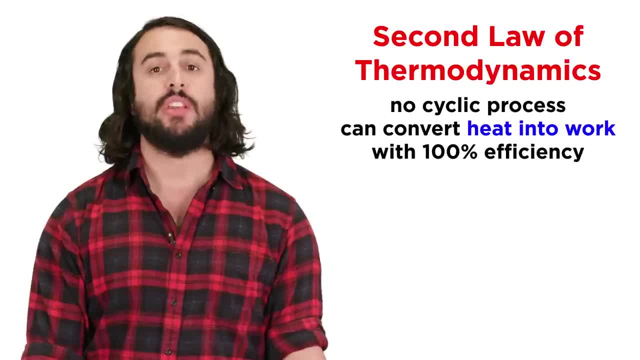 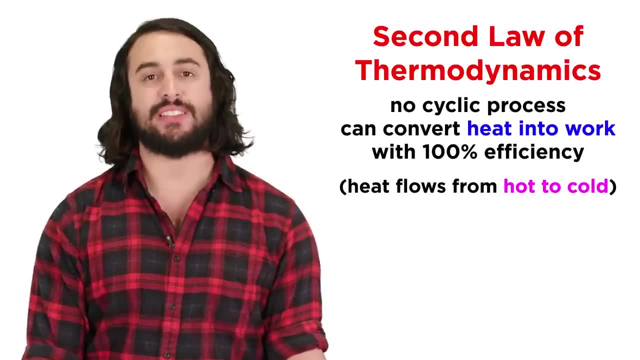 some quantity of heat entirely into work, Some of this heat will always be lost to the surroundings. This is a variation of another way of expressing the second law, which can also state that heat spontaneously flows from regions of high temperature to regions of low temperature. 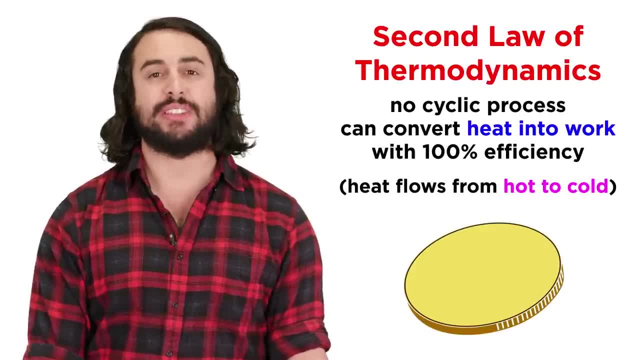 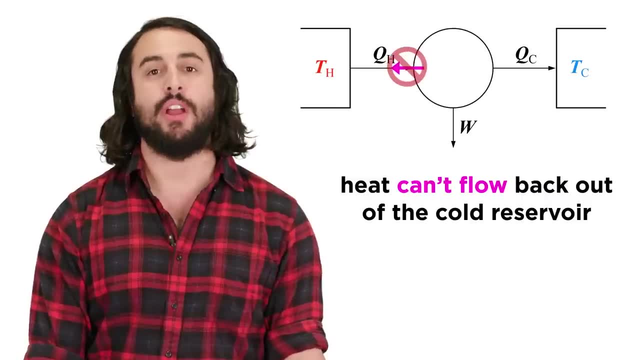 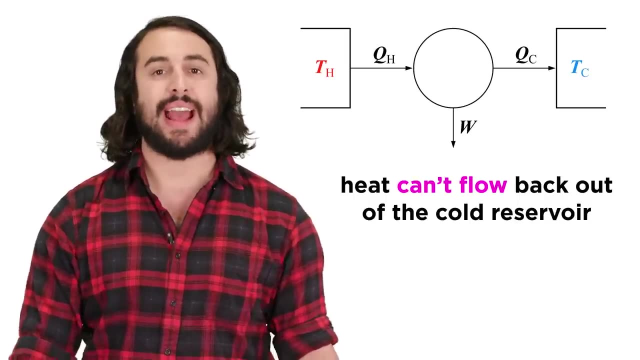 and not the other way around. These expressions can be considered two sides of the same coin, since heat therefore can't flow spontaneously from the cold reservoir to the hot reservoir of a heat engine, further supporting the idea that heat is always lost to the environment as the engine runs. 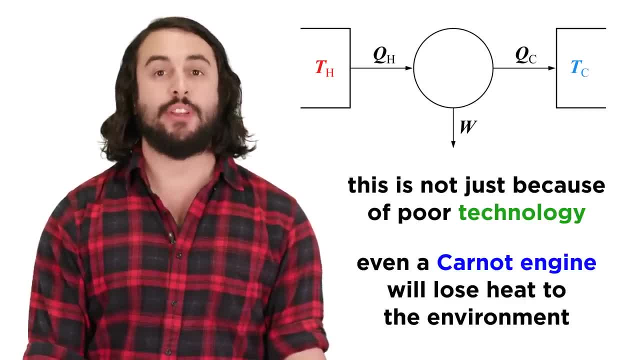 But this is not just a limitation of our technology. Even a purely hypothetical heat-saving process can be considered a limitation of our technology. Even a purely hypothetical heat-saving process can be considered a limitation of our technology. Even a purely hypothetical perfect heat engine called a Carnot engine can never operate. 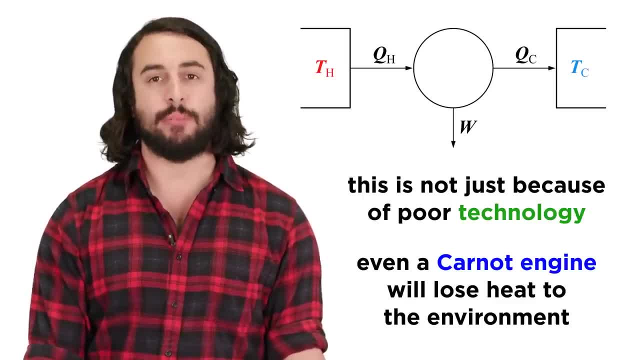 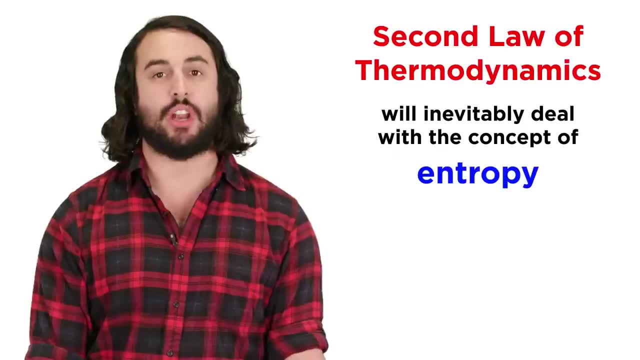 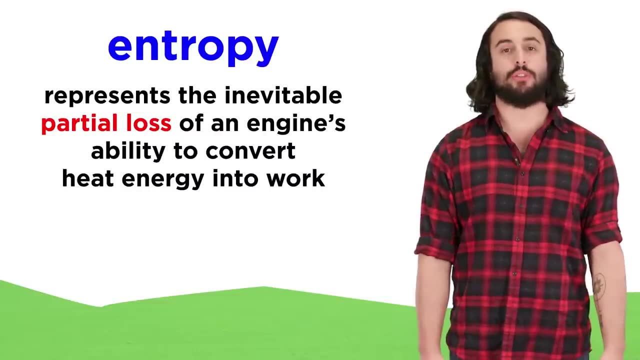 at 100% efficiency. This is a mathematical limitation of heat flow. Whichever way we choose to look at the second law, it will inevitably result in the discussion of a peculiar concept called entropy. Entropy is a term that represents the inevitable partial loss of a heat engine's ability. 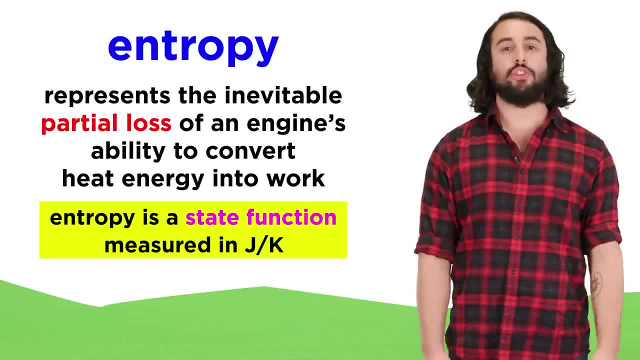 to do work. It is a state function measured in joules per kelvin, and it will be represented by a state function measured in joules per kelvin, and it will be represented by a state function which will be represented by the letter S. 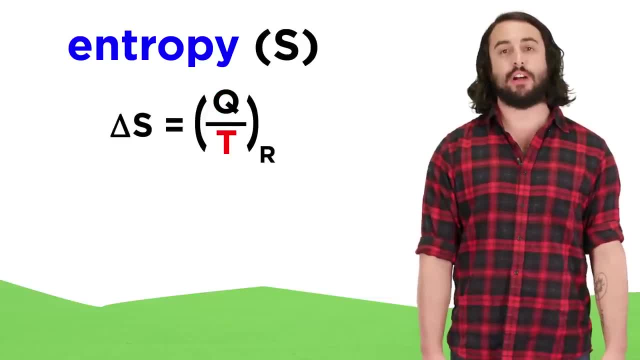 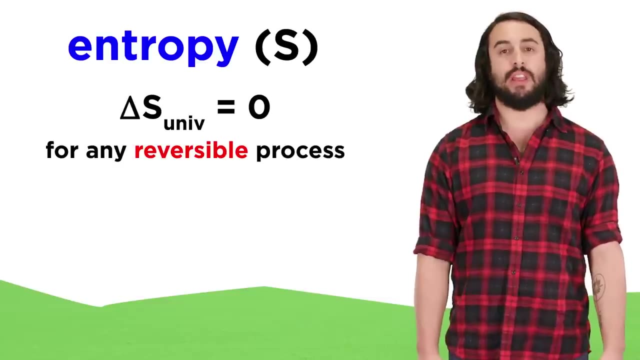 The change in entropy is given by heat over the kelvin temperature for a reversible process, and a mathematical ramification of this expression is that the change in entropy is zero. for a Carnot engine, This can be extended to say that the change in entropy of the universe will be zero for 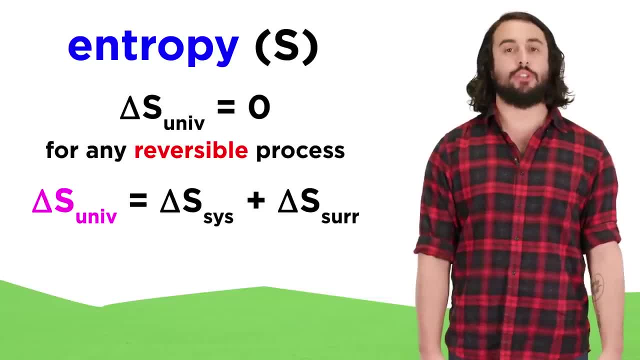 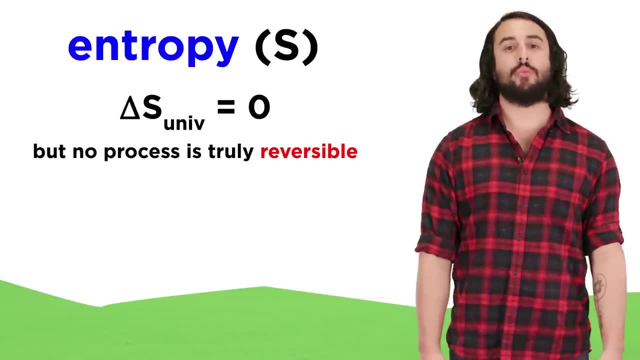 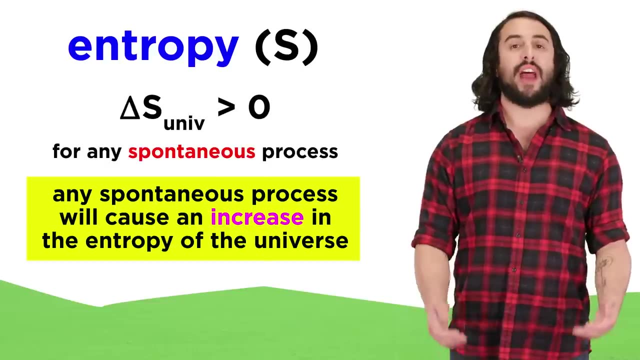 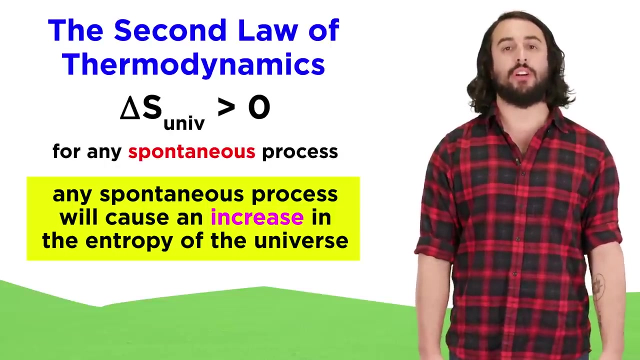 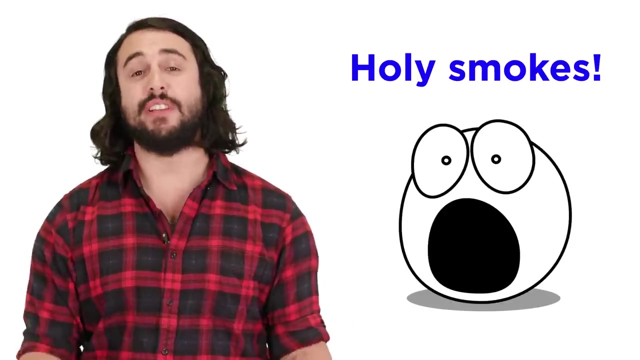 any reversible process, where the universe is understood to mean the system plus the surroundings. However, no process is truly reversible, So we should rather say that the change in entropy of the universe for any spontaneous process will be greater than zero, or that for any spontaneous processes, the entropy of the universe is 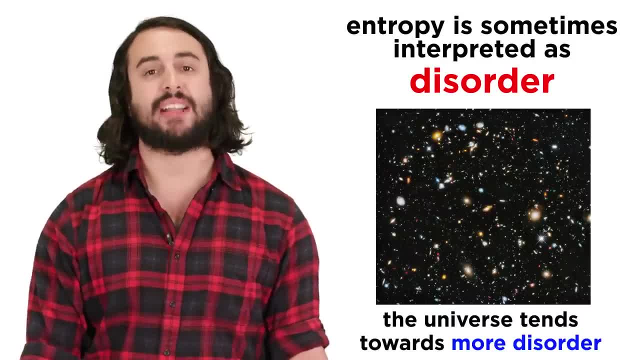 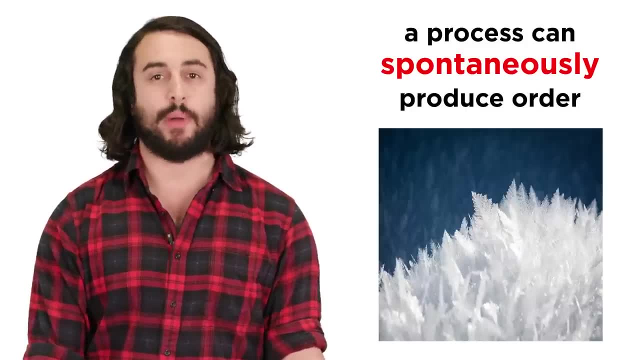 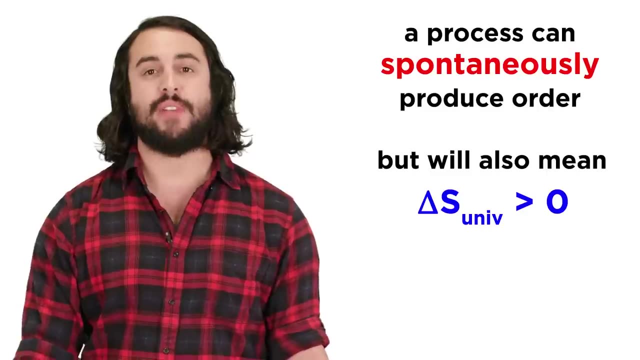 always increasing. It shows that the universe tends to move towards maximum disorder, and, while order can spontaneously form on the local level, like when water freezes to form ice or in the case of any living organism, this will always be accompanied by a dispersal of energy that increases the 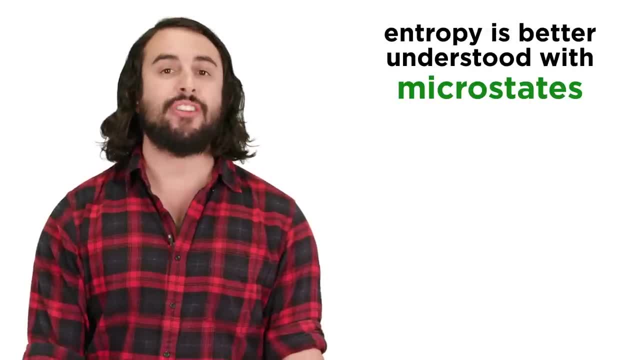 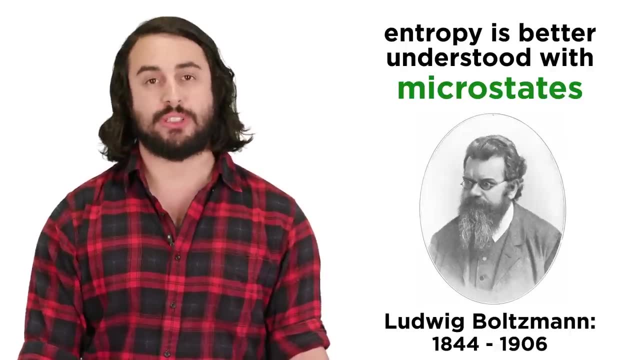 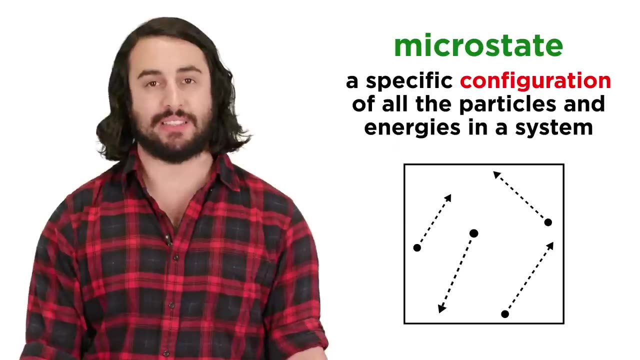 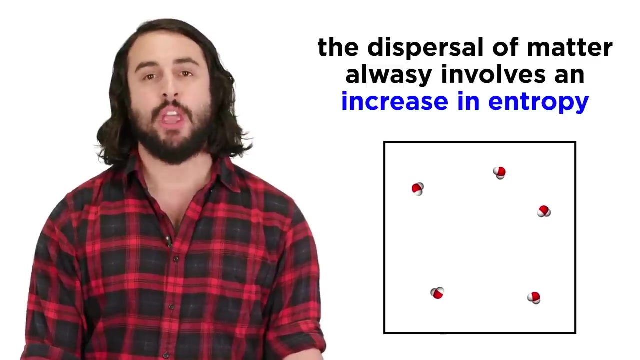 disorder of the universe as a whole. Entropy can be rationalized if we examine the concept of microstates introduced by Ludwig Boltzmann. A microstate is simply a specific configuration of all the particles and energies in a system. The dispersal of matter and energy, which is always accompanied by an increase in entropy. 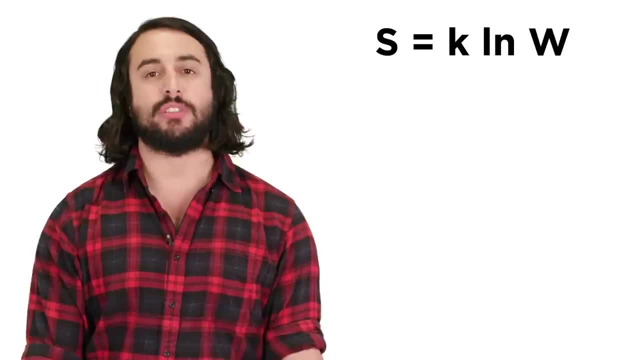 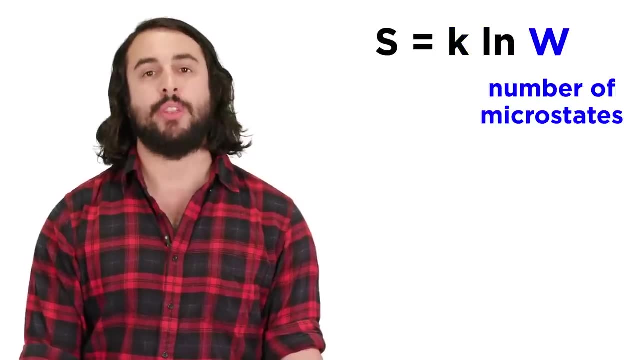 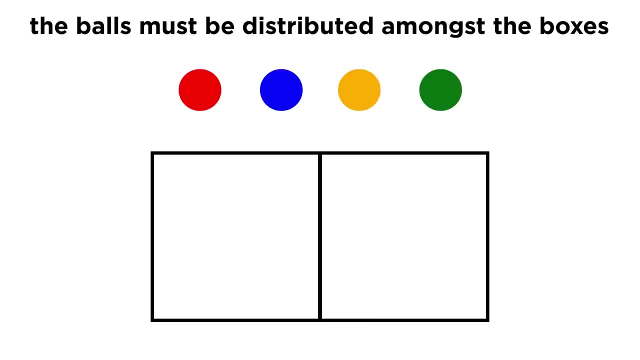 will tend to be spontaneous. Things move towards more disorder because of this equation. where S equals K, the Boltzmann constant times the natural log of W, where W is the number of microstates possible for a system. This is best understood with an example. 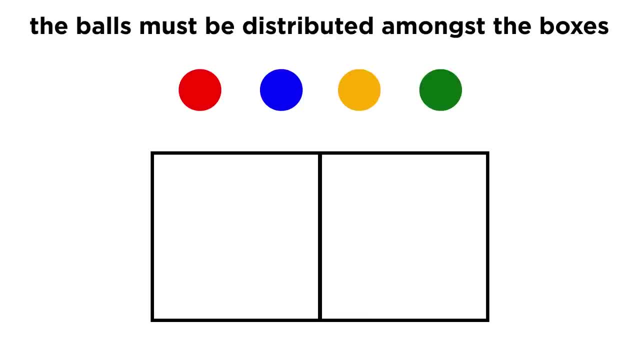 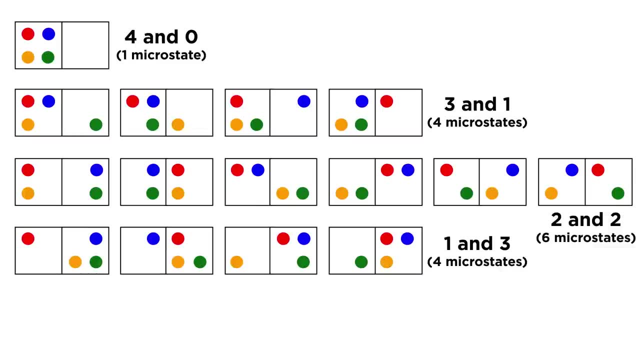 Say there are four balls to be distributed amongst two boxes. We could have all four in one, three in one and one in the other, two in two, one in three or all four in the second box. If these balls are all different colors, some distributions will contain a number of different. 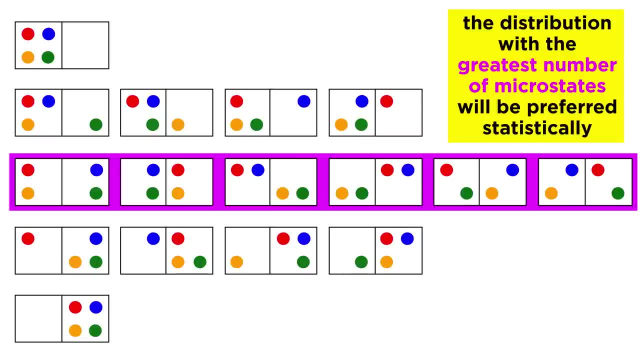 microstates, Statistical mechanics tells us that the most probable distribution will be the one with the most microstates, As in this case, the probability of finding the system in one of these microstates, with two and two, is six out of the sixteen total possible microstates.